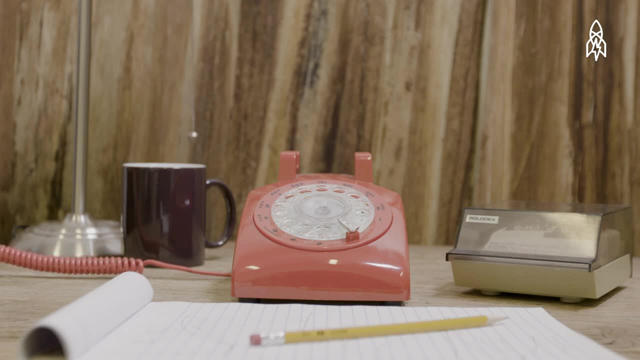 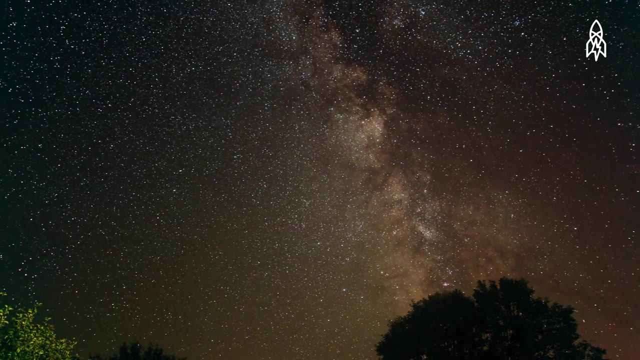 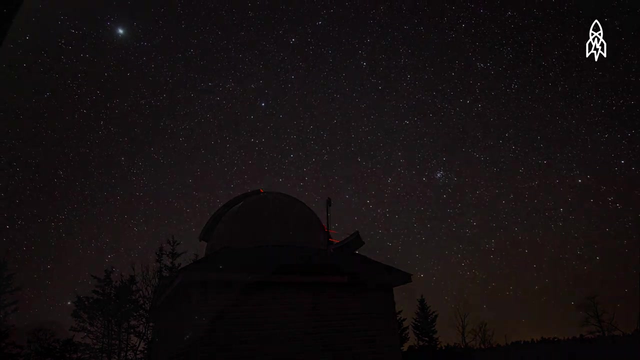 Dickey put the phone down and said: boys, we've been scooped. Robert and Arno had measured what Dickey and his team were searching for: The elusive cosmic microwave background radiation. He thought about a Big Bang source of the universe, realized that it would be very hot. 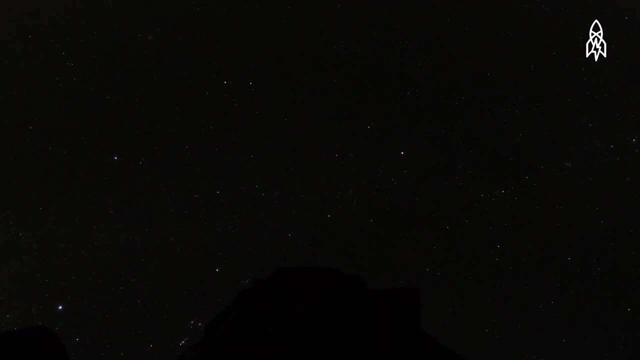 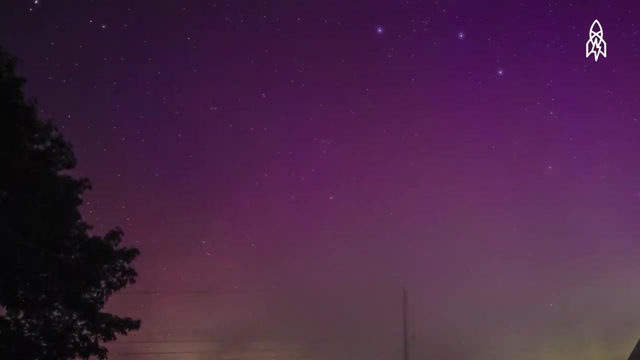 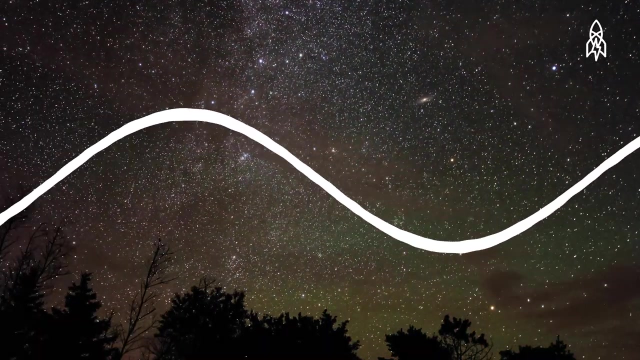 and therefore full of radiation. And as the universe expanded, that radiation would simply cool, And whereas it was extremely hot to start with, by now it would simply be microwaves. Now it's so cold that it would just be radio waves. 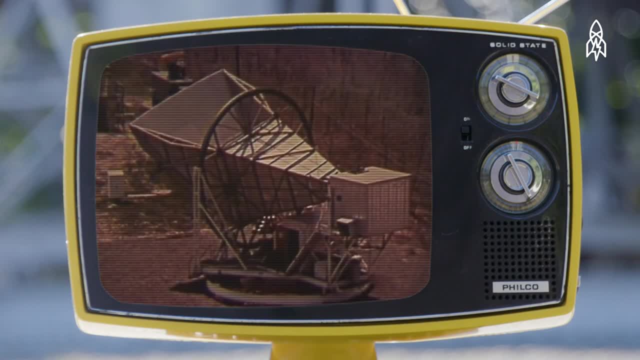 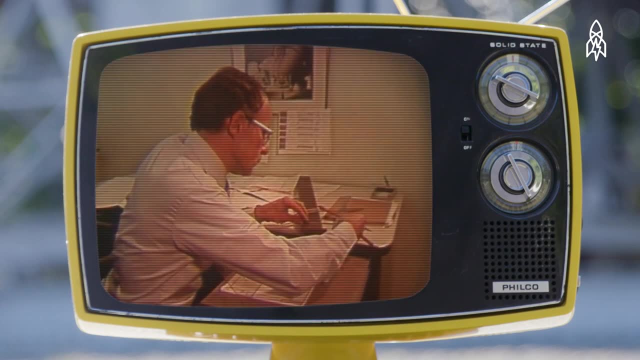 And this- not pigeons or the noisy city- was exactly what had been causing headaches for Robert Wilson and Arno Penzias. The two groups of researchers from Bell Labs in Princeton each wrote complementary research papers with their findings. They wrote one about the theory, we wrote one about our measurement and we published. 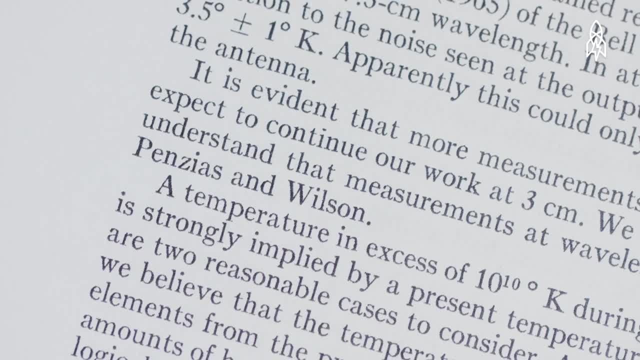 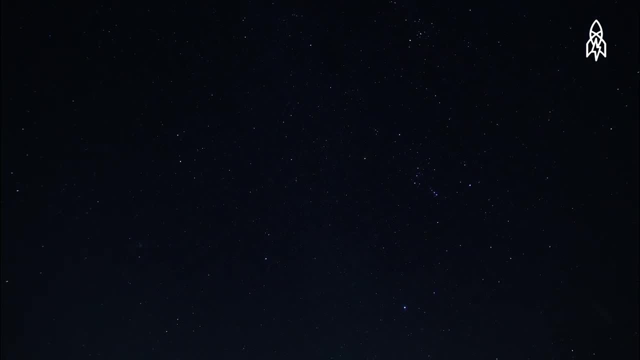 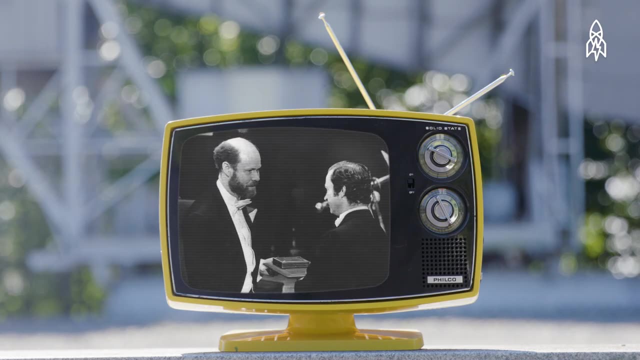 them. I think, unlike many changes that occur in science, there really was a paradigm shift. with very little pushback, It was huge. There was now evidence of a new theory for the beginning of the entire universe. Over a decade later, Robert Wilson and Arno Penzias were awarded the 1978 Nobel Prize. 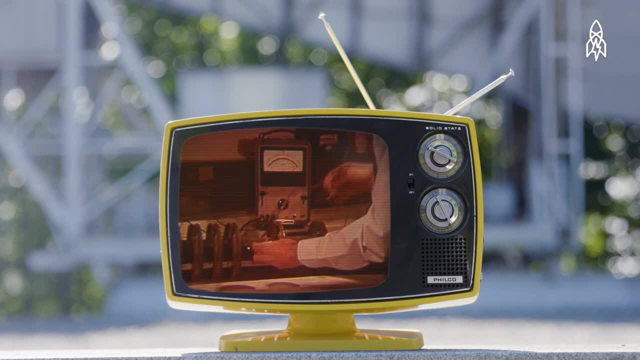 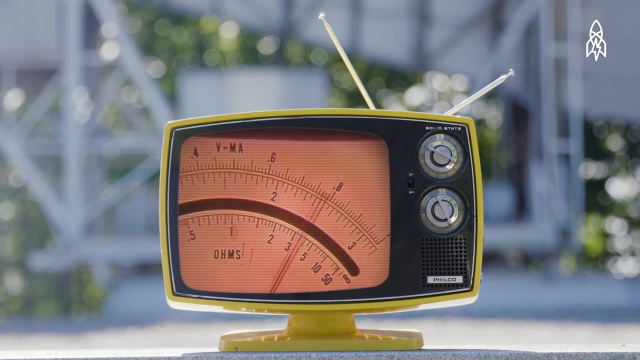 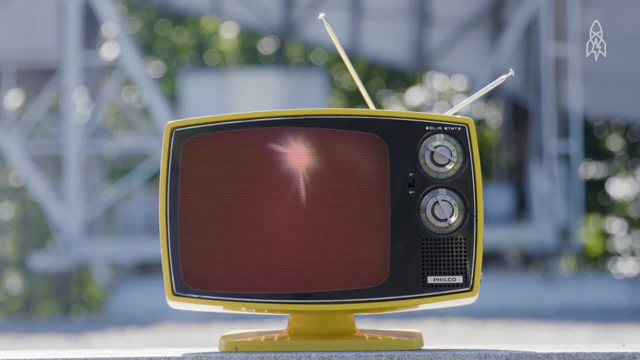 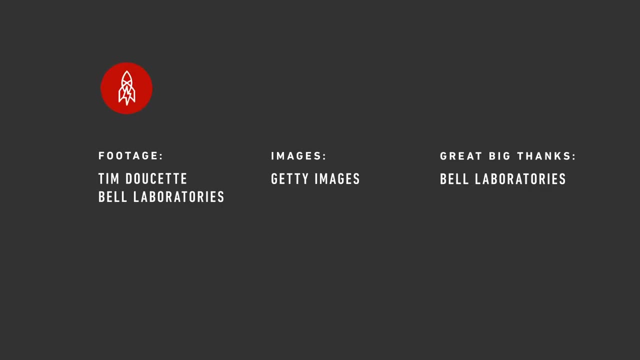 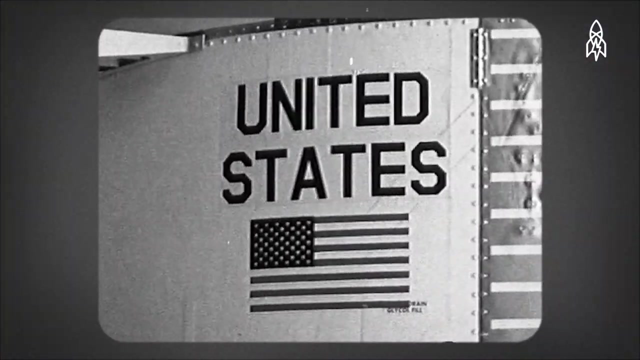 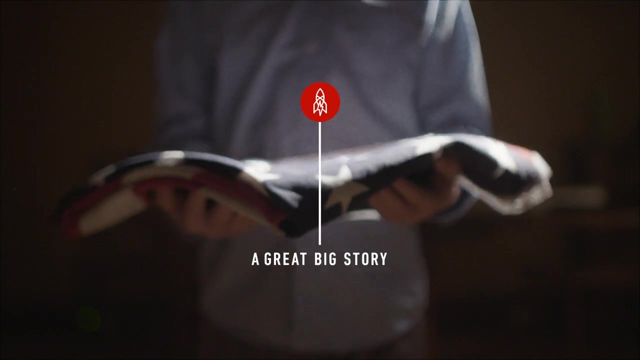 And it gives us our continuous picture of our own life And its endless degree of design, how it's transmitted and how it's organized diagnosis, and its endless degree of design how it's leaders about them in the study of science. It justHHHHH. 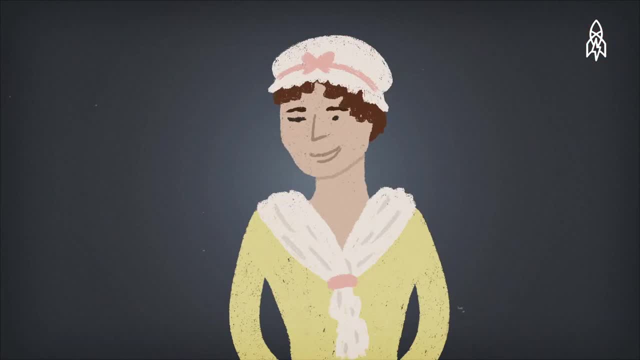 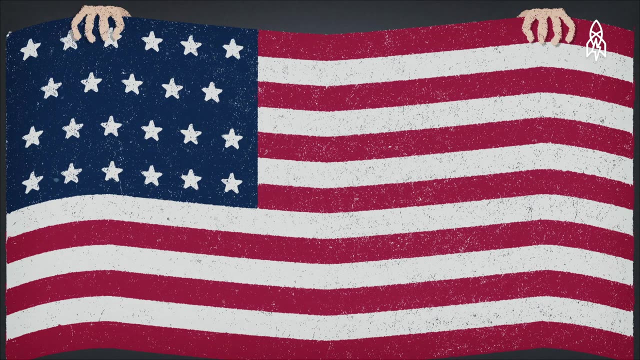 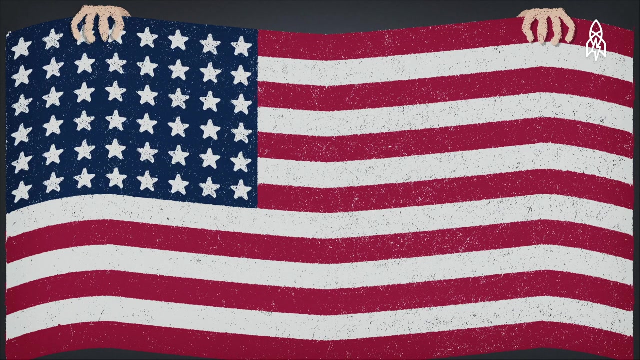 The American flag from 1776 was sewn by a lady named Betsy Ross. It had 13 stars in a circle representing America's original 13 states. As more states joined the Union, people kept adding more stars to the flag. So by 1958, the US flag had a total of 48 stars for the 48 states of that time. 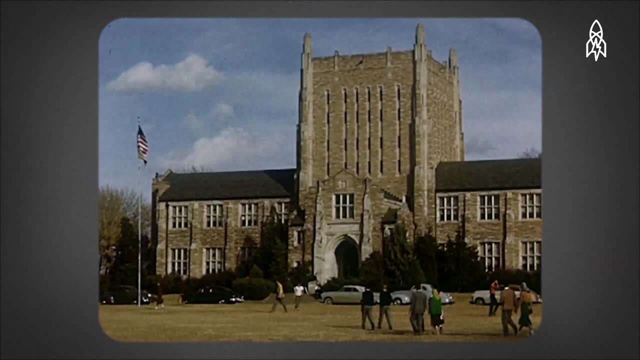 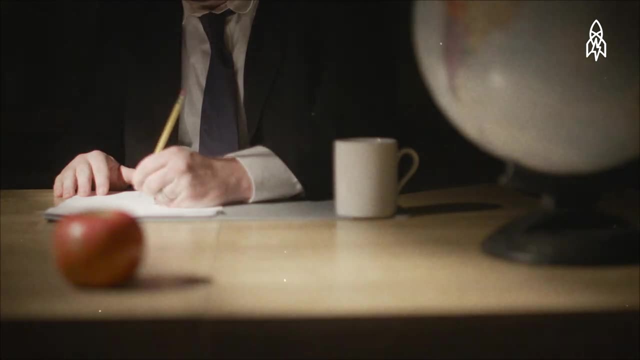 Which brings us to our high school student, Robert Heft. Robert's history teacher gave his students an open-ended assignment: Make a project illustrating your interest in American history. It could be anything. So, Robert, who was jazzed about hearing that Alaska and Hawaii were going to become states? 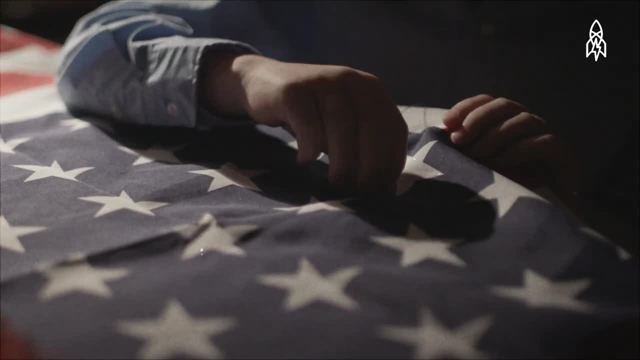 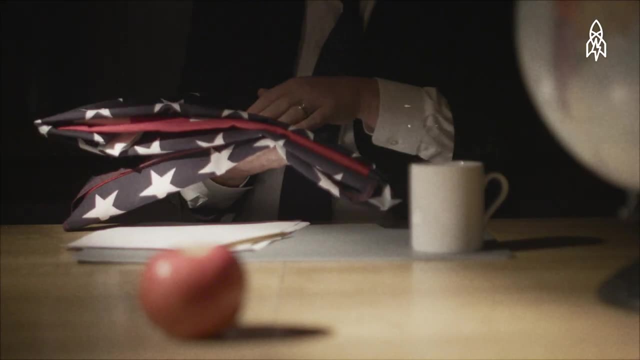 cut up an old 48-state flag in his grandparents' basement and designed his own vision for a 50-state flag. When he turned in his final assignment, Robert's teacher said: Anyone can make a flag And it's got the wrong number of stars. 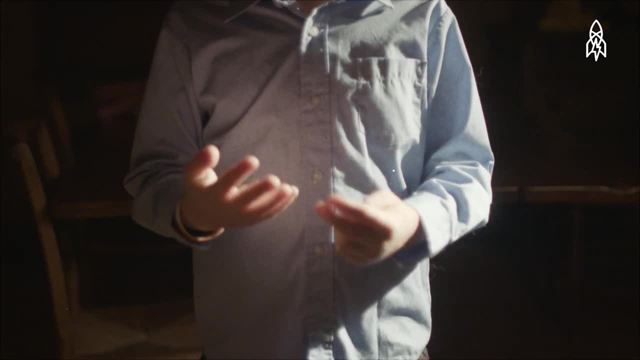 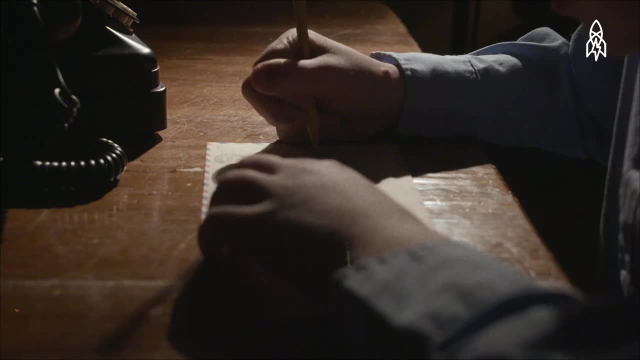 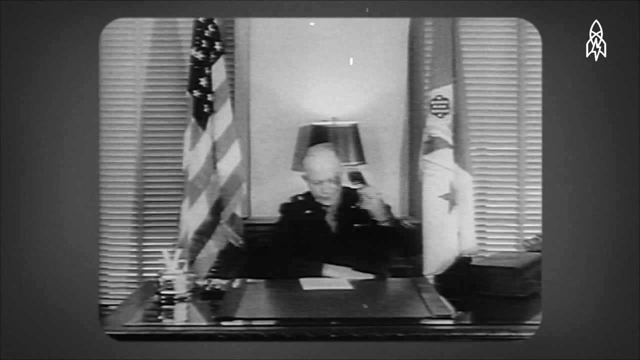 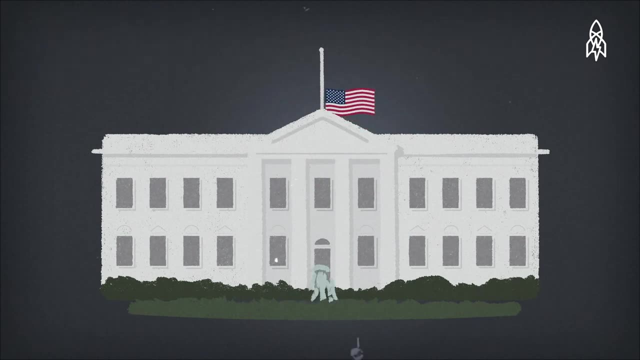 phone rang. Hello, Hello, Robert Heft. It was President Eisenhower with news that Robert's 50-state flag design had actually been chosen as the new official flag of the United States. The President invited Robert to Washington where he saw his American flag fly for the. 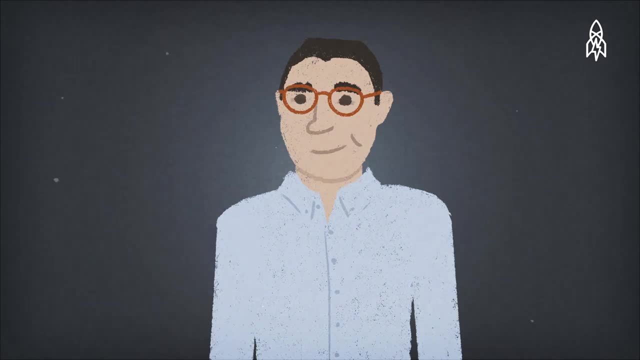 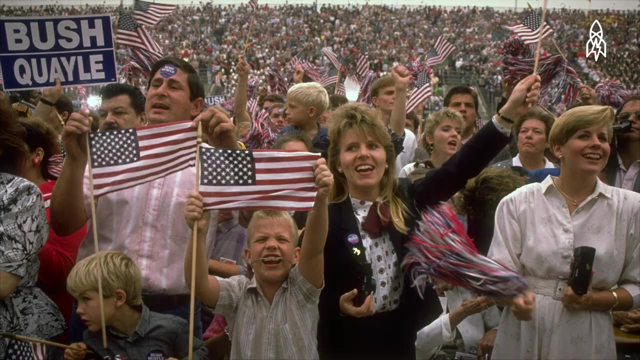 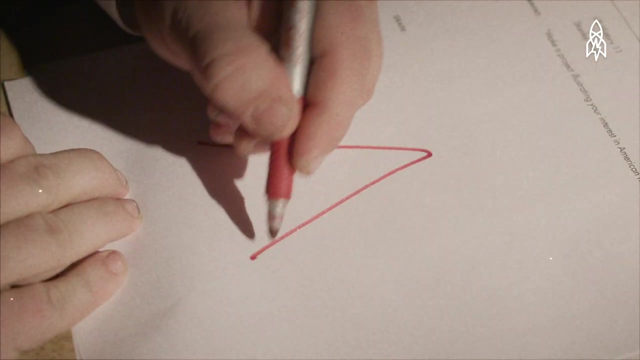 first time on July 4th 1967.. Since then, Robert's 50-state flag has remained unmatched as the quintessential symbol of America. But I know what you're thinking. Whatever happened to that B- Robert's teacher honored his promise and changed the grade to an A. 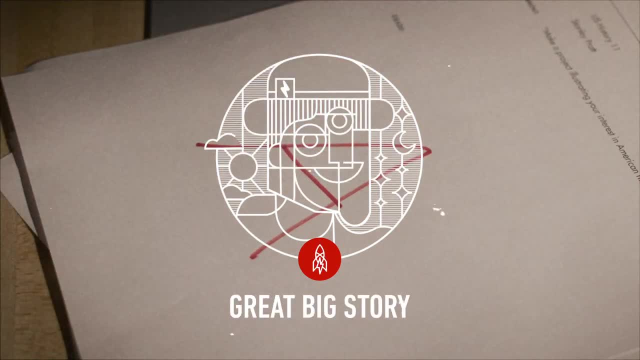 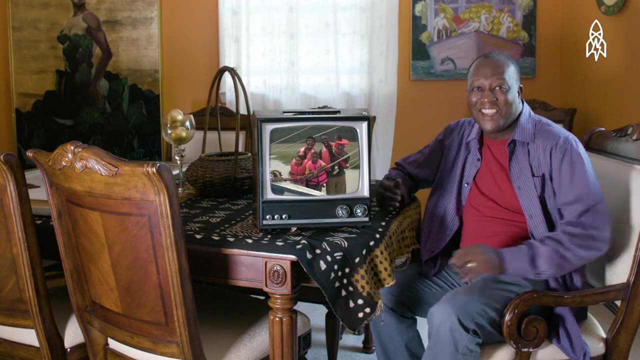 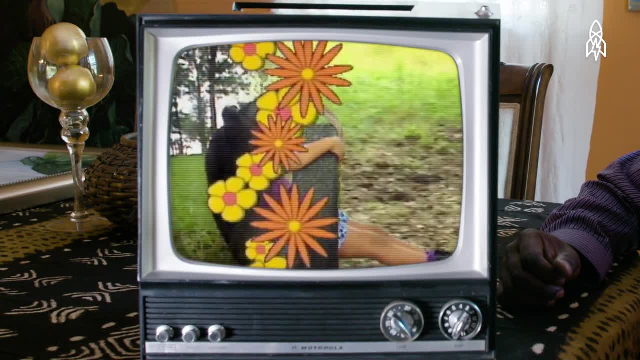 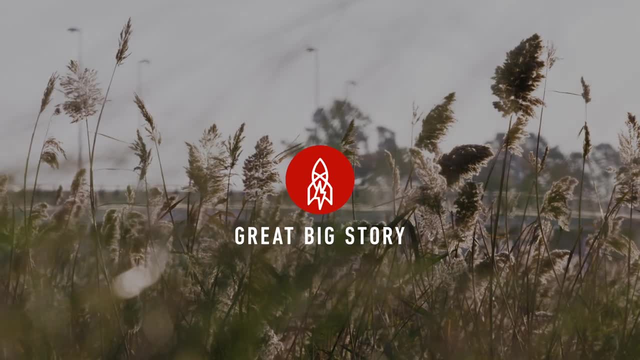 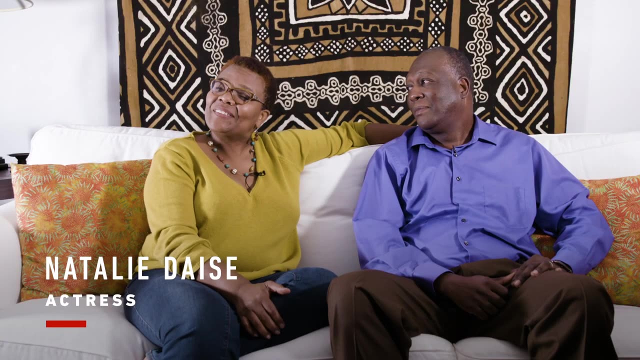 Well, it's a real place kind of. Well, it's a real place kind of. I'm Natalie Days and I played Miss Natalie on Gullah Gullah, Ireland. My name is Ron Days and I served as a dad. 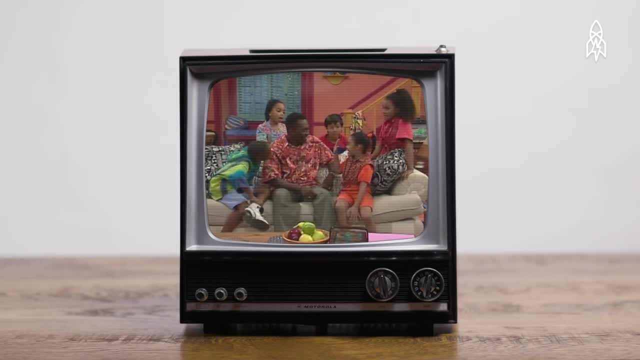 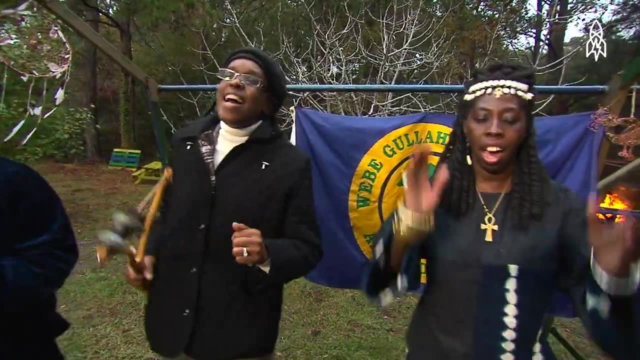 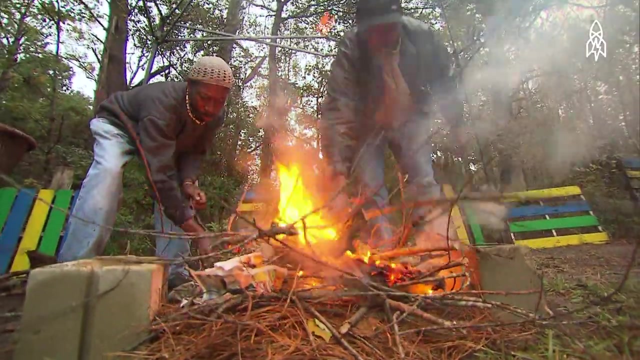 Show me how old you are, Shailene Five. There is no real place named Gullah Gullah Ireland, except on TV. Really, Yeah, on the Gullah Geechee culture which was passed on by enslaved West Africans who were brought. 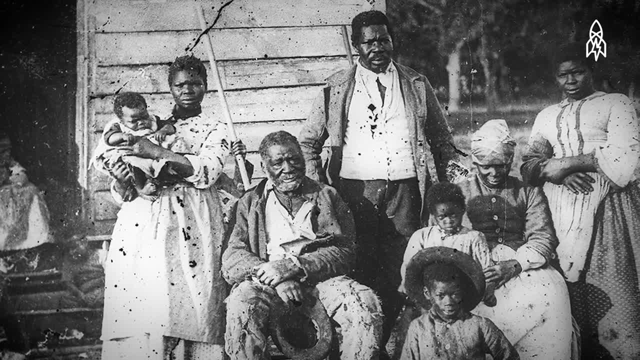 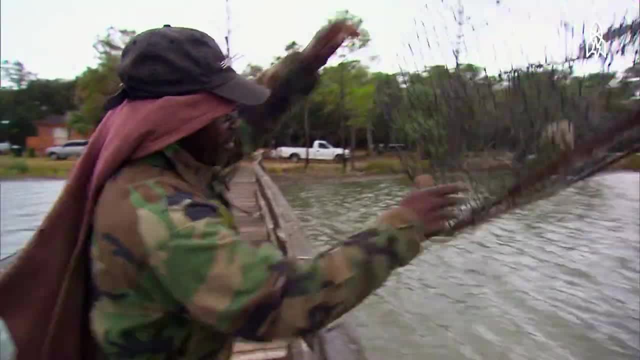 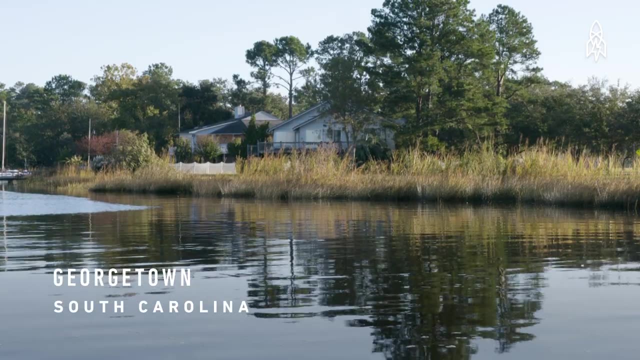 to this country. Gullah Geechee culture was born out of several African cultures and languages brought here by enslaved people. Everything from cuisines and traditional practices have been maintained through generations of settlement in coastal villages in Georgia and the Carolinas. I am Gullah Geechee and proud of it. 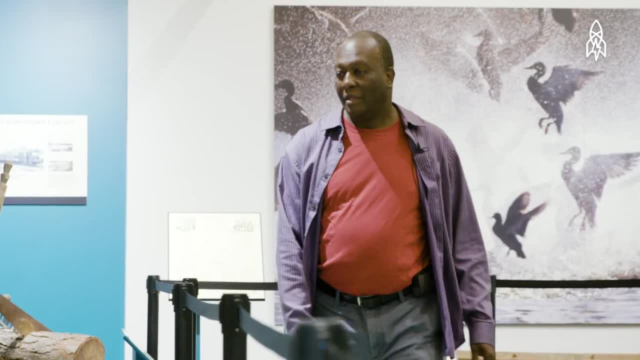 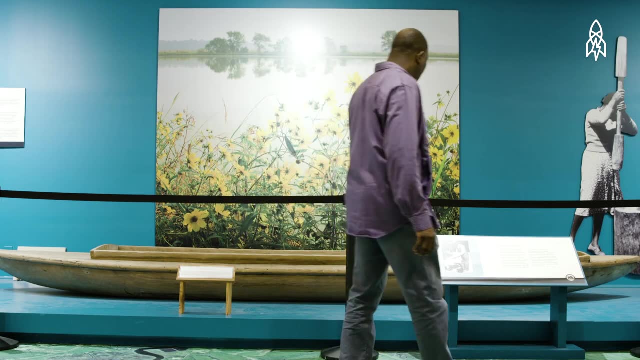 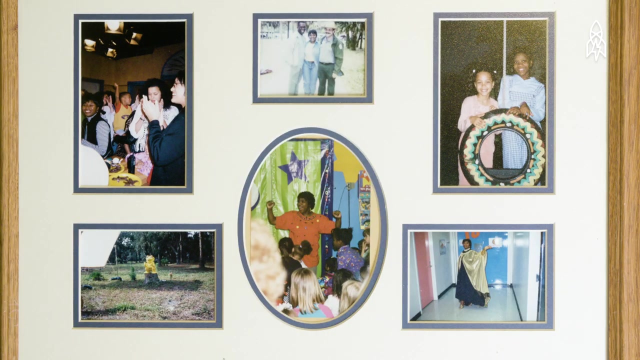 It's important to me to make sure that Gullah Geechee culture is preserved, because it's a very important factor of American cultural heritage. When Natalie and Ron got the opportunity to present their culture on TV, they jumped at the chance. By the time we met the woman who became the executive producer, we had been traveling. 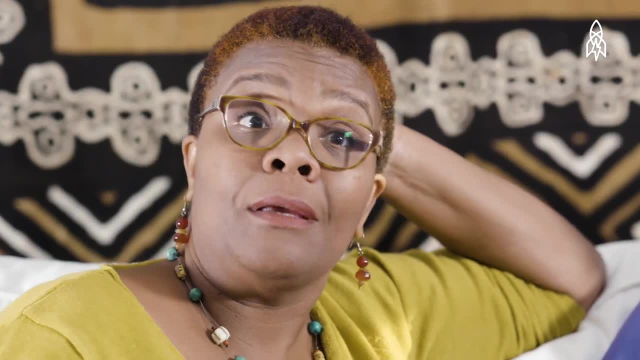 around the country doing stories and songs of Gullah culture. That's what we did In the beginning. we didn't know that it was so significant. There had never been an event like this. We had never done a show like that before. 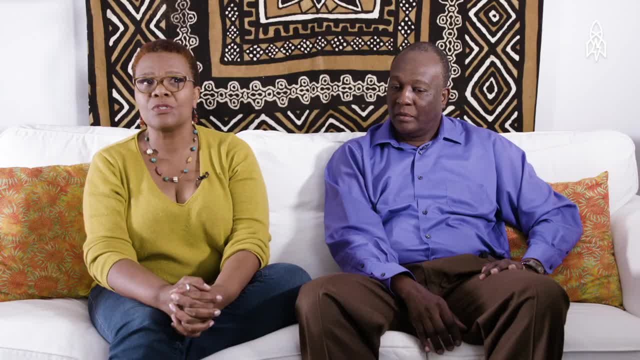 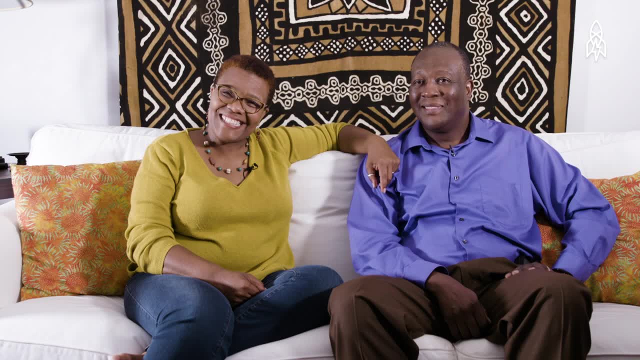 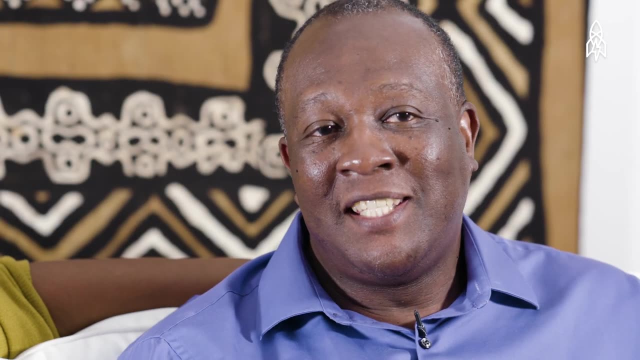 We wanted a show where our children could see themselves. We actually ended up with a show where everybody could see themselves in us. Before we go, would you guys mind singing us out? Man, we get asked that a lot. Come and let's play together in the bright, sunny weather. 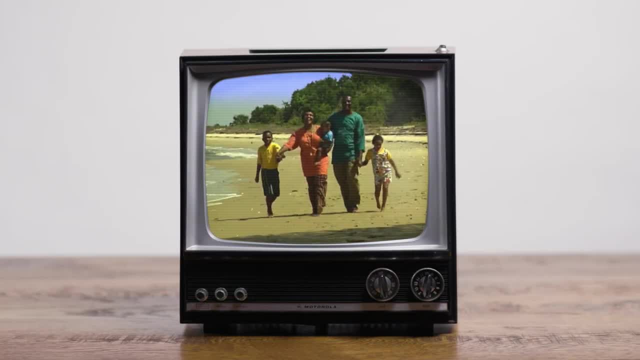 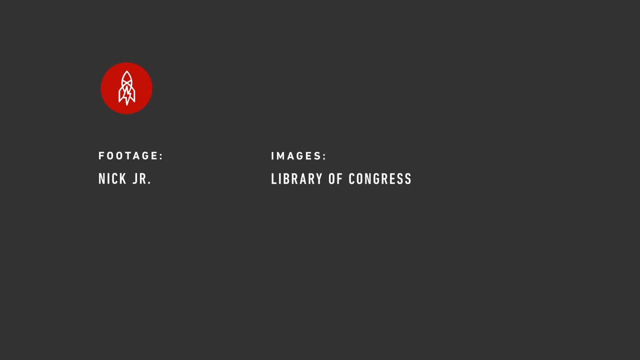 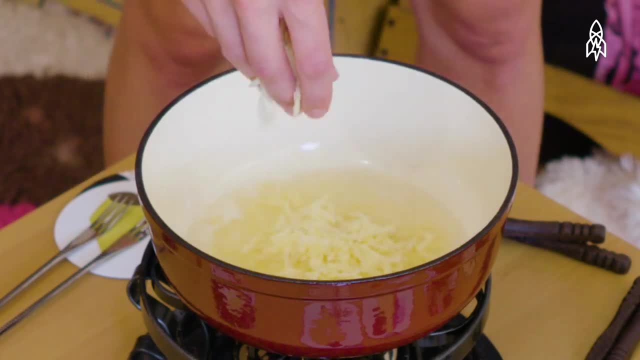 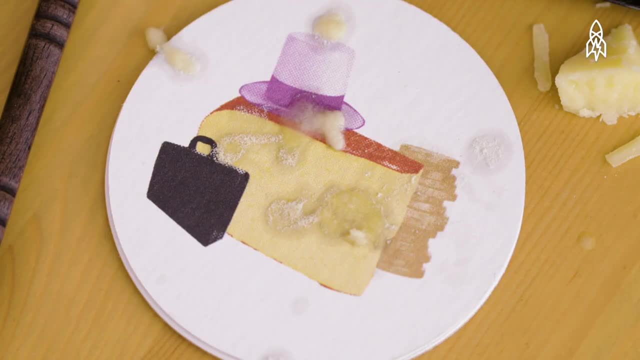 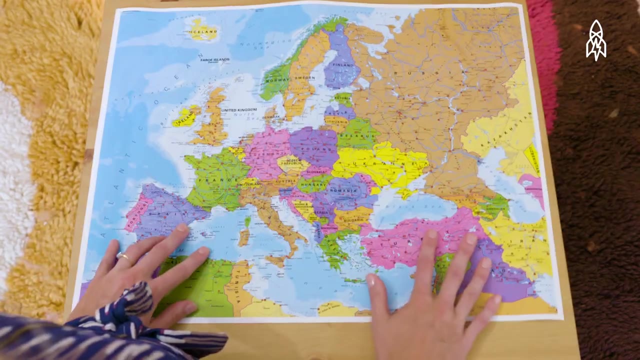 But that didn't just happen by chance. There was an ominous force behind it, A real-life cheese cartel. A hundred years ago, cheese was a hot commodity in Switzerland. It was exported at high volumes and fast volumes and played a major role in the Swiss economy. But that all changed after World War I. European countries, devastated by the war, could no longer afford to buy expensive imported cheese, which was bad news for Switzerland. So the government stepped in and they formed the Cheese Union. Basically it was a cartel and it worked like this: 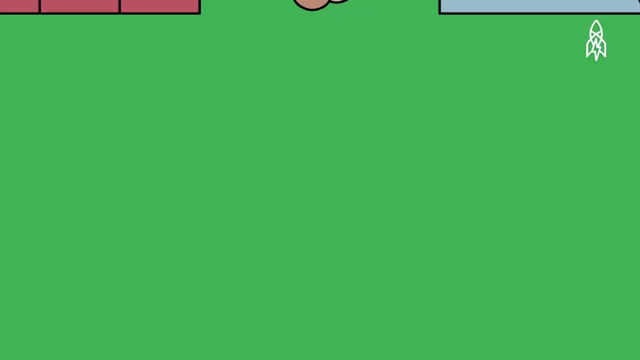 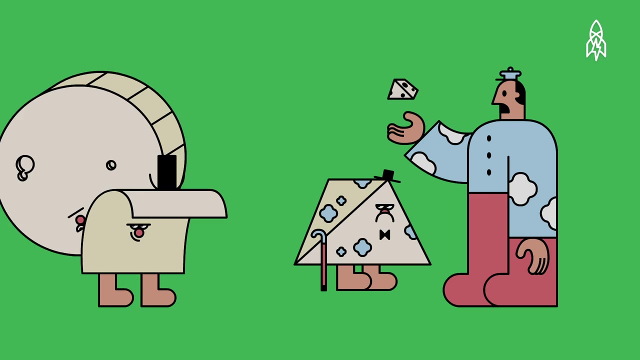 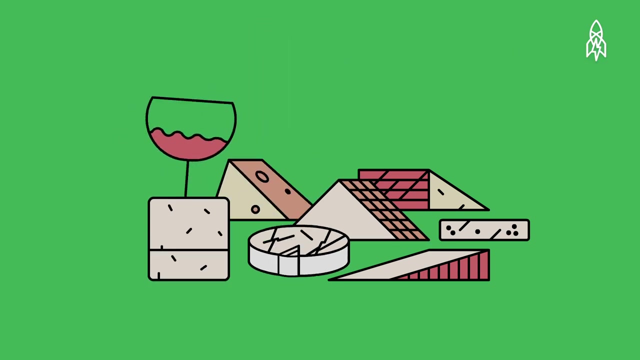 The first thing they did was force every dairy farmer and cheesemonger to fix the price of cheese, eliminating competition, meaning everyone could stay in the game. The cheese cartel also told them exactly how much cheese to make and limited the varieties. So, instead of making thousands of different kinds of cheese, they only made seven, And it worked. The cartel controlled the cheese supply for decades. By the 70s they got greedy and wanted to expand their cheese racket globally. So they introduced the world to a dish already popular in the freezing cold Alps fondue. 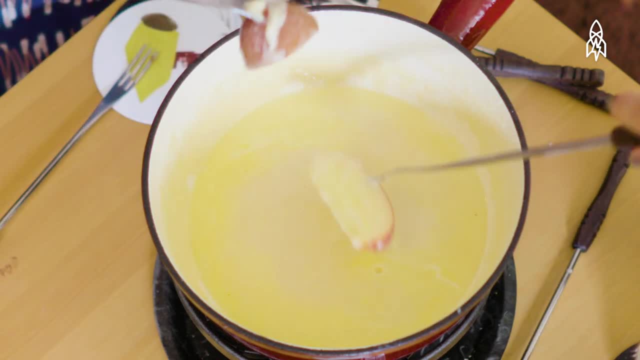 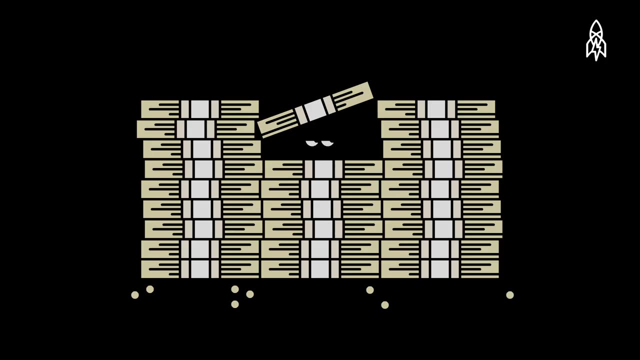 By marketing cheese for fondue, the cartel was able to sell more. I mean, think about it. It takes a lot, and I mean a lot of cheese to fill a pot. But as with most cartels, things got shady. 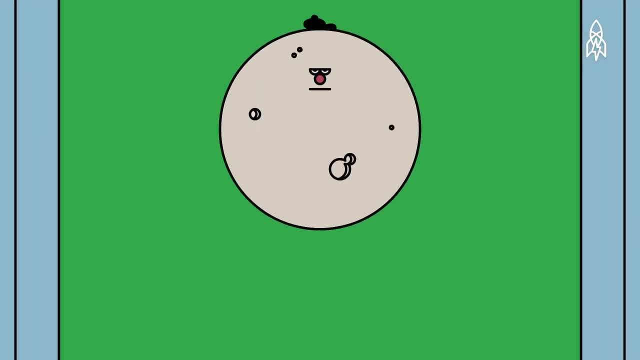 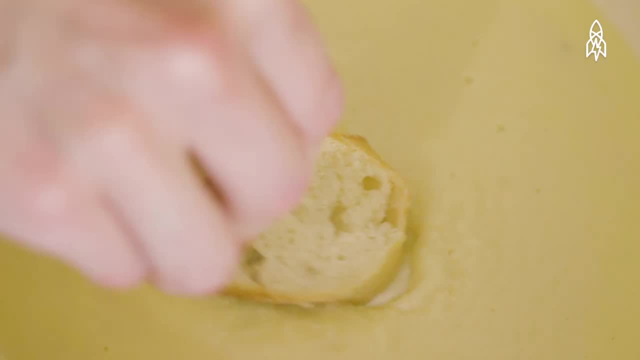 Money went missing, people went to jail and by the 1990s the Swiss Cheese Union was dismantled. So there you have it. The reason we know and love fondue is because of a shady government program that convinced the world to consume. 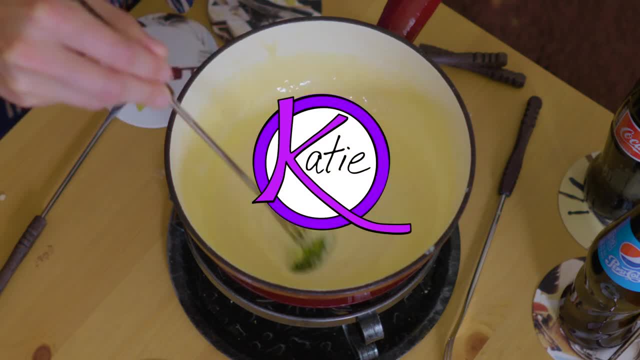 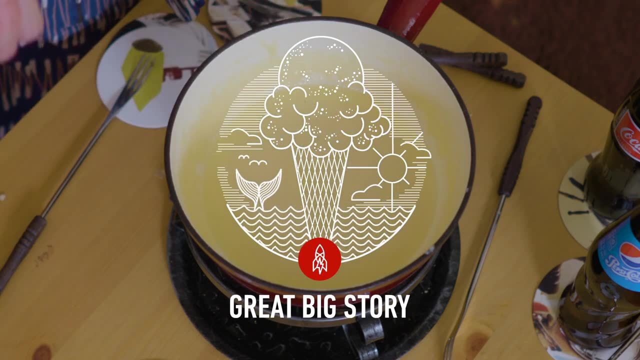 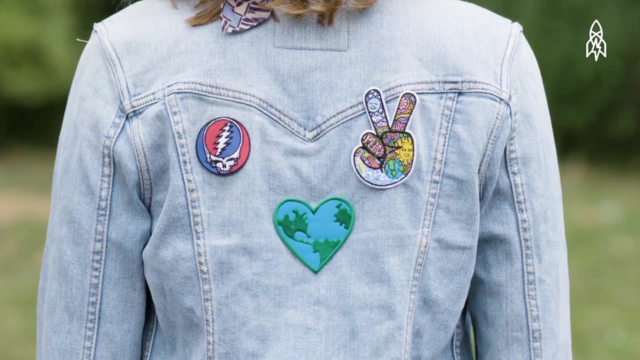 massive amounts of melted cheese. LTC. THE HIPPY CREED- HIPPY CREED, The National Littering. The Channel B-H-I-P-P. The Channel The Wish, The Max, The S-H-I-L-E. The National Littering, The National Littering. 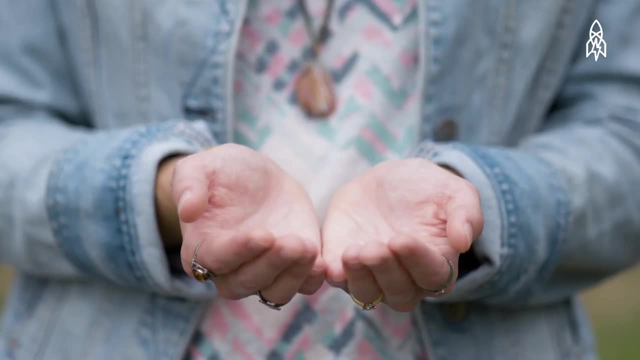 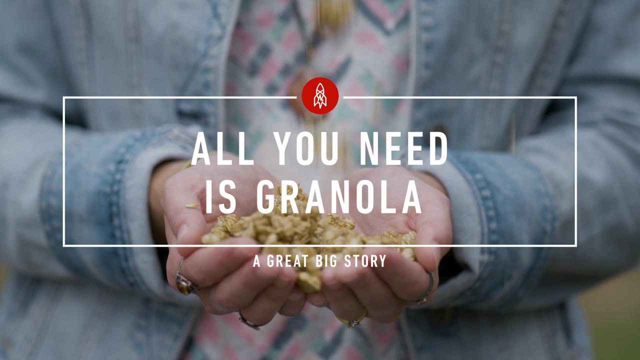 Peace, love and rock and roll. It's the hippie creed, along with some flour power and some crunchy granola. And we call hippies crunchy granola because of, well… Granola: The link between the people, the culture and the granola. 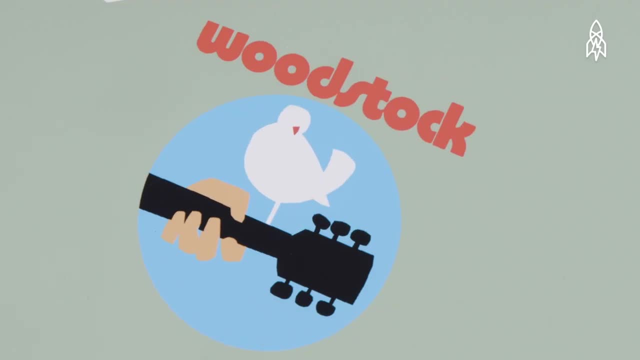 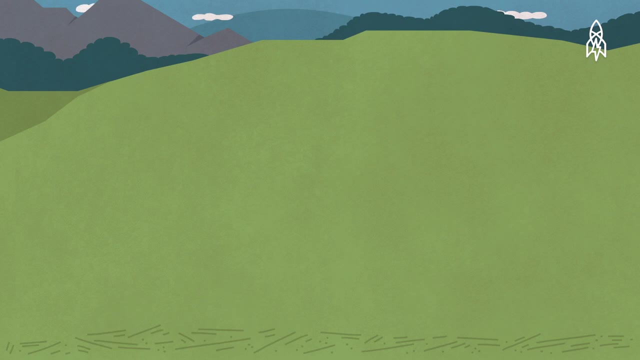 It started in 1969 at Woodstock. Organizers estimated that 200,000 fun-loving people would fill the small town of Bethlehem, New York, for the three-day historic festival, But the number of attending doubled and the next thing they knew. there were over 400,000 people camping out, which led to shortages, food shortages, And well, that left the munchies-craving, furry-loving hippies a little hangry. This is where the savior Hugh Romney came in. 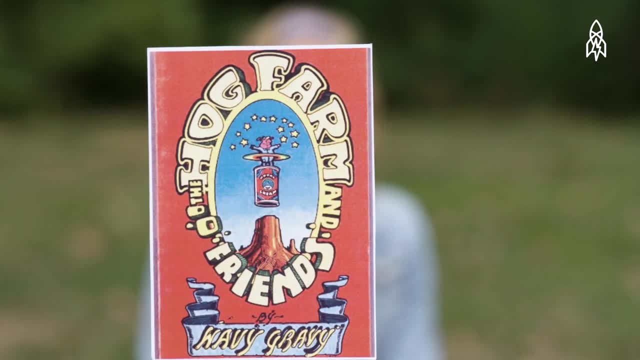 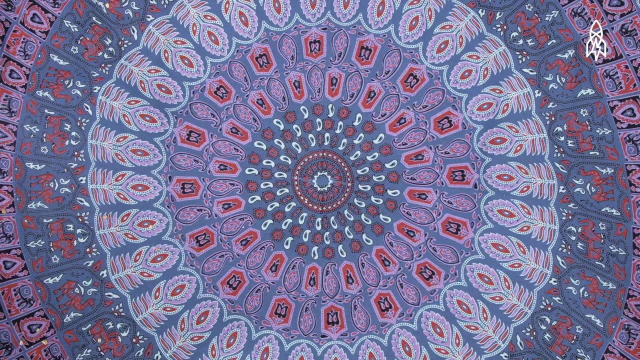 Hugh and his commune Hog Farm were hired to help organizers run the festival. Upon seeing the food shortage, they stepped in to help. They rounded up a group of volunteers, hit the streets and came back with- you guessed it- granola. 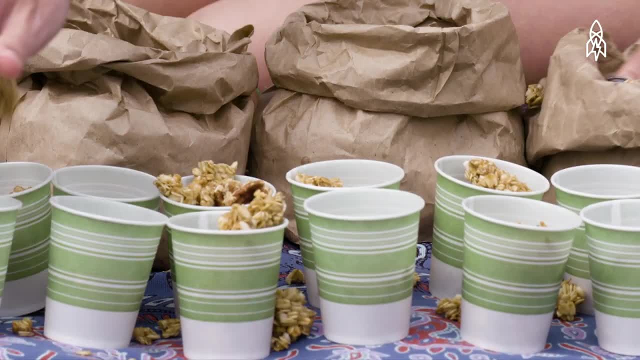 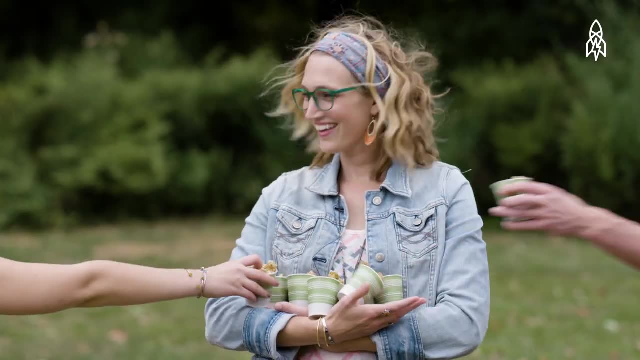 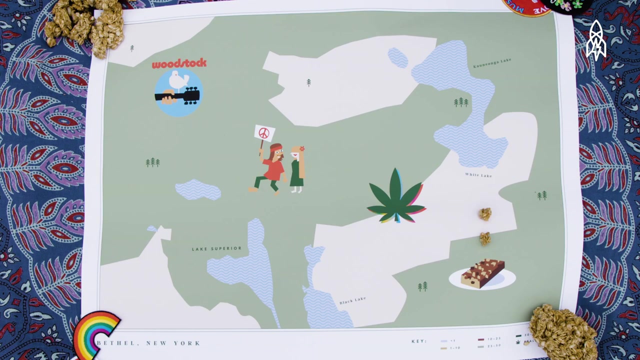 Members of Hog Farm filled tons of cups and Hugh took the stage and announced there would be breakfast in bed for 400,000.. The hippies ate it up And for many it was their first introduction to the crunchy stuff. And so there you have it, the original bond.